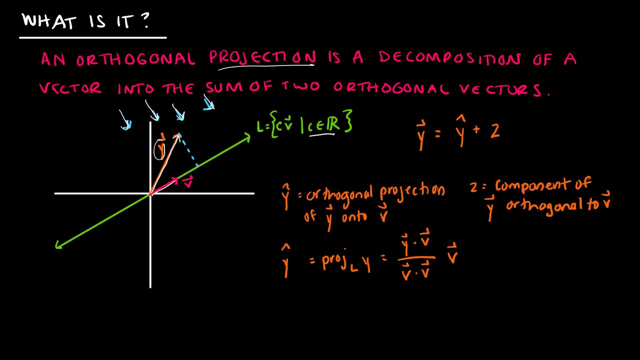 to line l and I'm looking at the shadow that y would create. that's essentially what I'm doing, Is I'm looking to write y as a sum of some scalar multiple of v and then that distance from y to v. that is orthogonal or that is a right angle. So we have some different notation here. 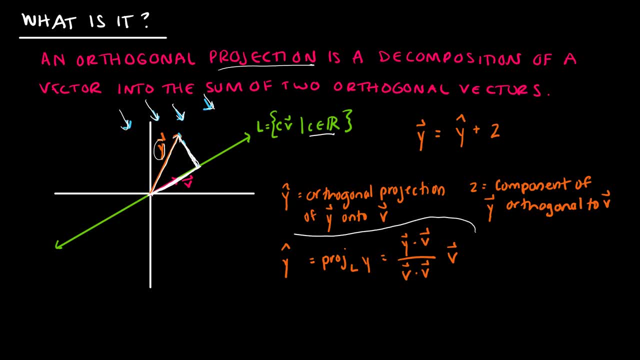 and really there's only one formula and that is how to determine y hat, y hat, which is the projection of y onto l, and again that has to do with dot products. So I'm going to take y times the vector, the dot or the dot product of y in the vector over the dot product of the vector. 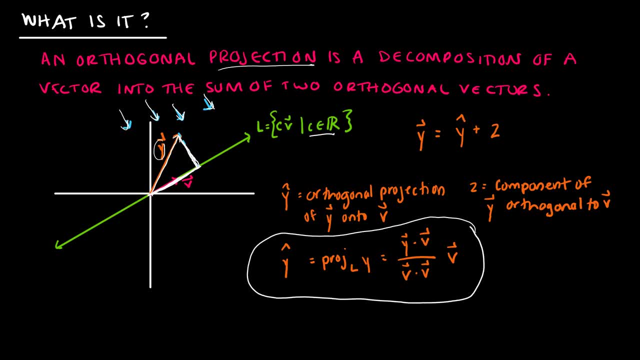 and itself multiplied by the vector. So this is not going to make any sense until we actually do a question. but before we start a process of, you know, actually finding an orthogonal projection, I wanted you to get an idea of what we're doing. So again, we have this vector y, we want to write it. 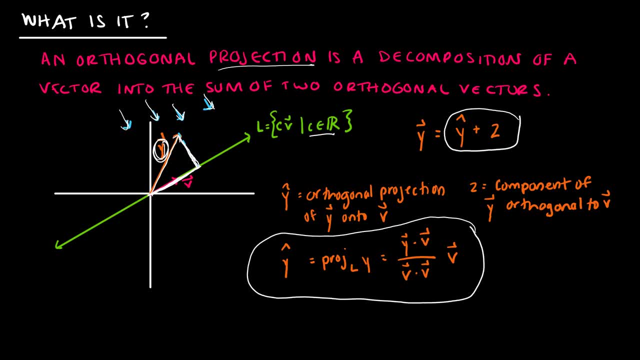 as the sum of two orthogonal vectors, so two vectors that are at a right angle to one another, and so that would be some scalar multiple of v plus some vector that is orthogonal to v. So let's take a look at how we'll actually go about doing this. 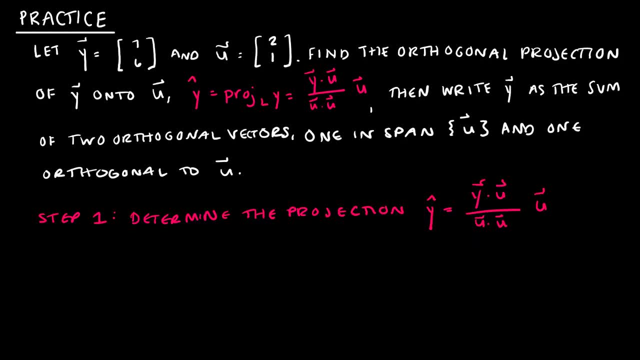 We're going to do this practice question together, step by step, and again I tried to write it out- exactly what we would do or the process that we would do. So what we're looking for the first thing is we have two vectors and I want to find the orthogonal projection of y onto u. 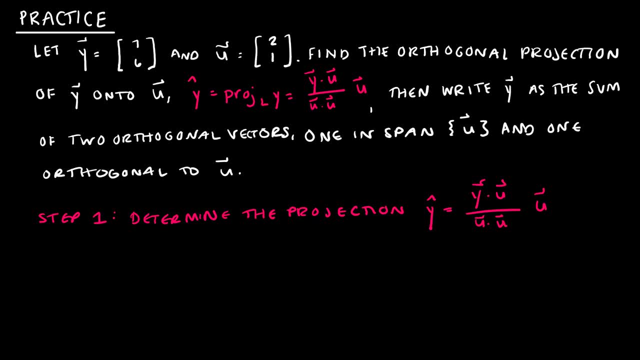 So again, if you think about that last slide u, would be that vector v was the vector on my last slide. So I'm looking at that line that would be created by u and say what would that projection of y look like if we were to add a vector that was at a right angle to u? So again, 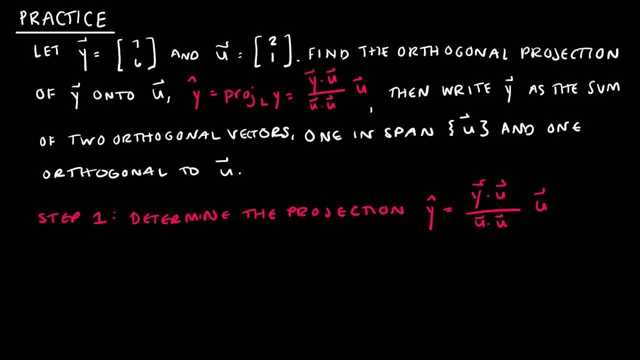 if there were some ray of light shining perpendicularly to u, what would y look like projected onto that line? And again, this one's easy to determine because we are just looking at a formula. So y hat, which is a projection, is found by taking the inner product. 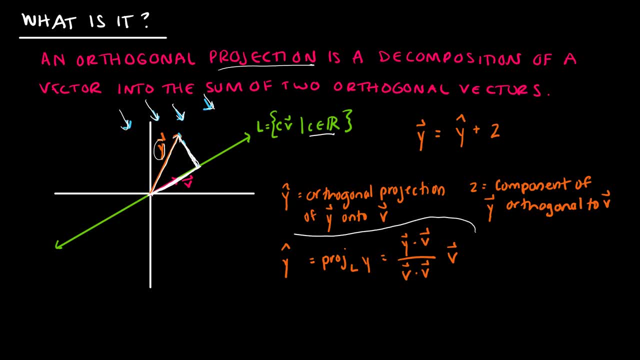 and really there's only one formula and that is how to determine y hat, y hat, which is the projection of y onto l, and again that has to do with dot products. So I'm going to take y times the vector, the dot or the dot product of y in the vector over the dot product of the vector. 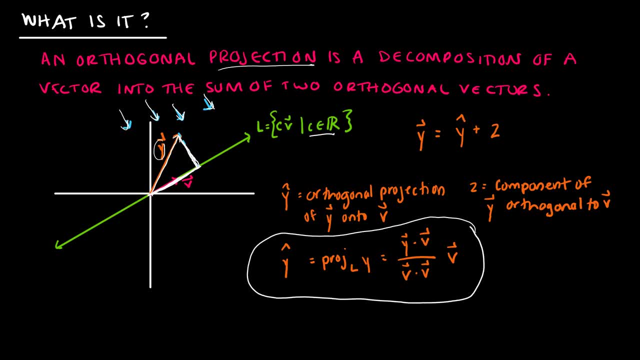 and itself multiplied by the vector. So this is not going to make any sense until we actually do a question. but before we start a process of, you know, actually finding an orthogonal projection, I wanted you to get an idea of what we're doing. So again, we have this vector y, we want to write it. 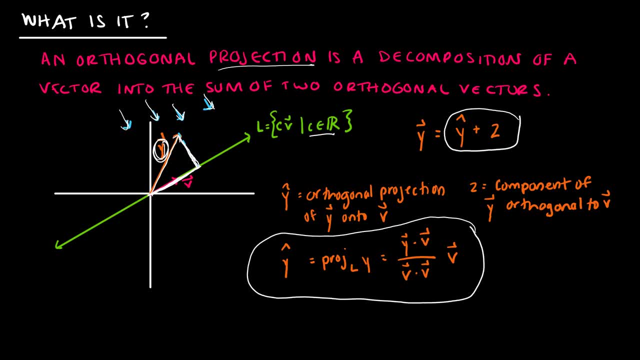 as the sum of two orthogonal vectors, so two vectors that are at a right angle to one another, and so that would be some scalar multiple of v plus some vector that is orthogonal to v. So let's take a look at how we'll actually go about doing this. 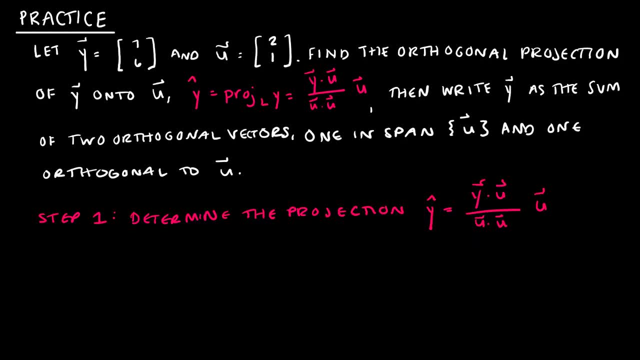 We're going to do this practice question together, step by step, and again I tried to write it out- exactly what we would do or the process that we would do. So what we're looking for the first thing is we have two vectors and I want to find the orthogonal projection of y onto u. 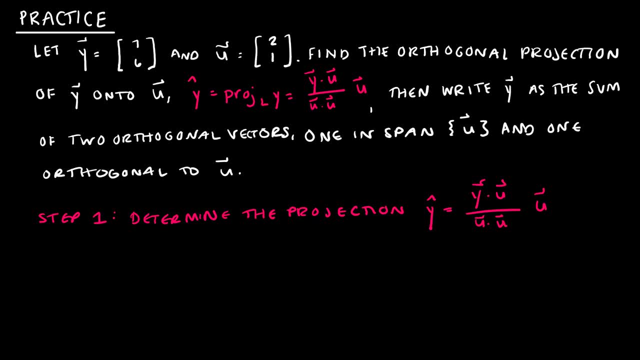 So again, if you think about that last slide u, would be that vector v was the vector on my last slide. so I'm looking at that line that would be created by u and say what would that projection of y look like if we tried to do this practice question together, step by step, And again? 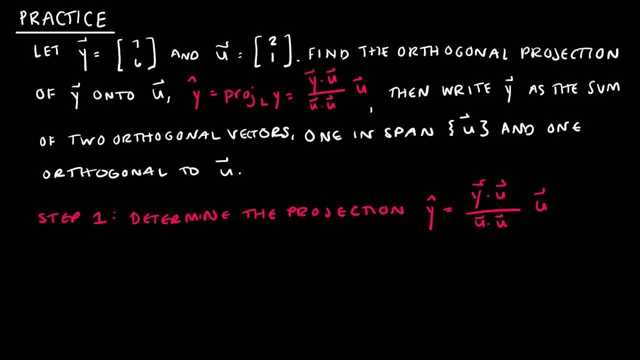 if there were some ray of light shining perpendicularly to u, what would y look like projected onto that line? And again, this one's easy to determine because we are just looking at a formula. So y hat, which is a projection, is found by taking the inner product. 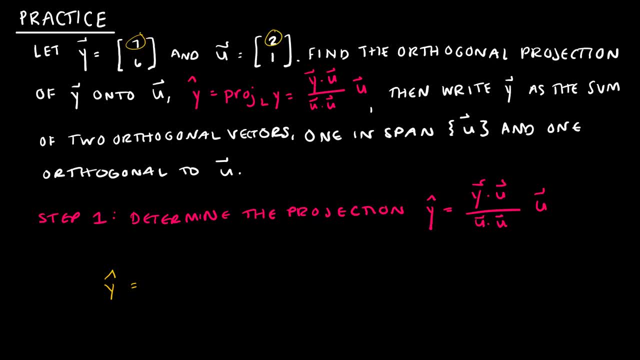 of y and u. so that's 7 times 2, or 14,, plus 6 times 1, or 6, over the inner product of u with itself. So that's 2 times 2,, which is 4,, and 1 times 1,, which is 1.. And that's going to be. 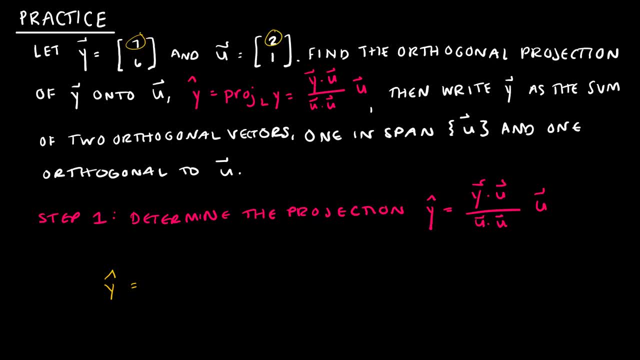 of y and u. so that's 7 times 2, or 14,, plus 6 times 1, or 6, over the inner product of u with itself. So that's 2 times 2,, which is 4,, and 1 times 1,, which is 1.. And that's going to be. 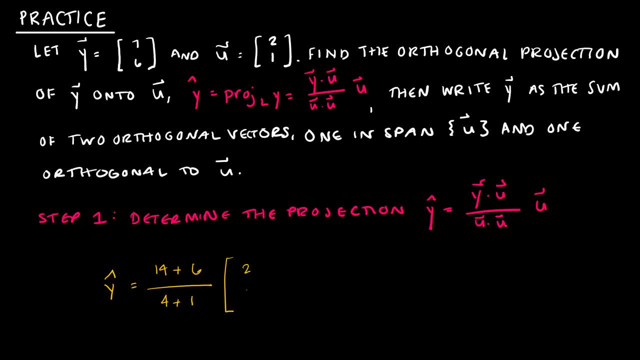 taken times vector u, which means I have whoops, I have 20 over 5 times vector u, which means 20 over 5 is 4 times vector u. So my projection is 8, 4.. So again, 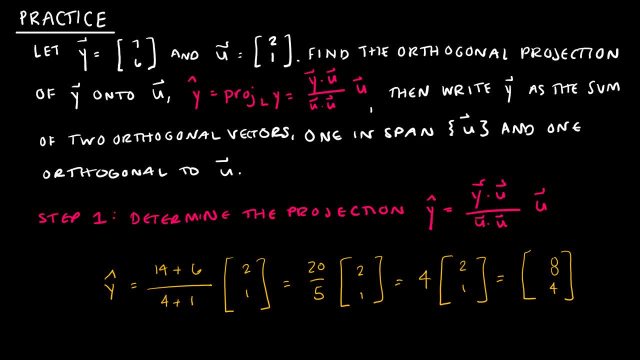 if you were to graph that, you would be looking at 7,, 6, and the line created by all of the scalar multiples of u, along the line created by 2,, 1, which obviously 8, 4 is on that line, And obviously 8, 4 is on that line And so that's going to be taken times vector u, which means 20 over 5, is 4 times vector u, So my projection is 8, 4.. So again, if you were to graph that you 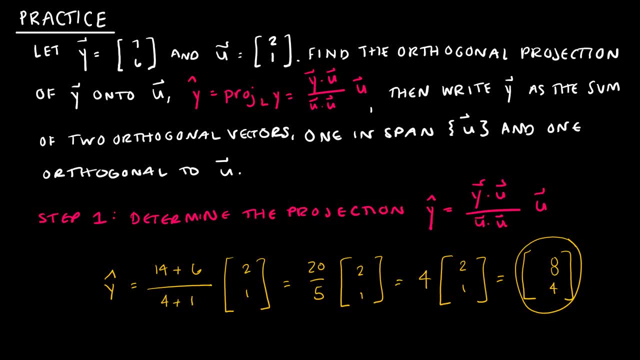 would be looking at 7,, 6, and the line created by all of the scalar multiples of u along the line. That is where y would sort of land if we were looking at the projection of y onto that line. Step two, then, is to find the component, which is what I would add to the vector that I just 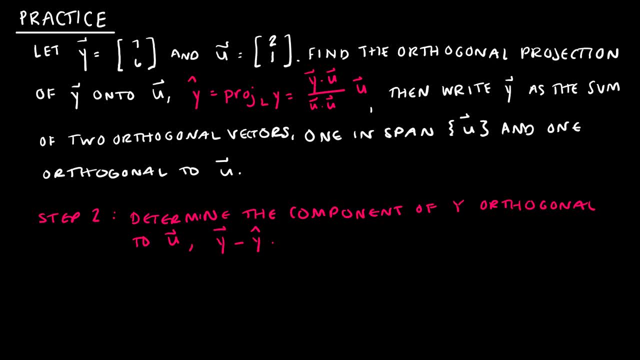 found in my last question, or last part of the question, so that I can write y as the sum of two orthogonal vectors. So one is in span u. Well, that's the one we just found. So, if you'll recall, I just found that the sum of two orthogonal vectors is the sum of two orthogonal vectors. 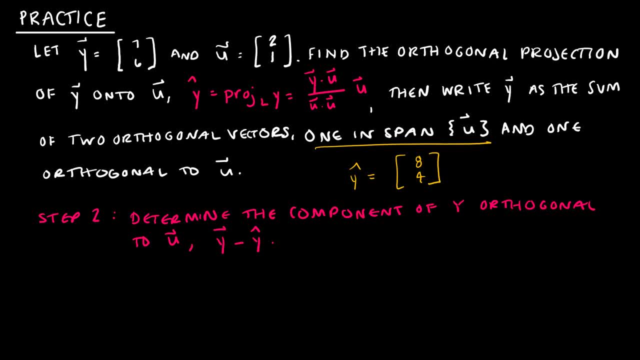 I just found that y hat was 8, 4.. And if I had a coordinate plane here- 1,, 2,, 3,, 4,, 5,, 6,, 7,, 8,- 1,, 2,, 3,, 4,, 8, 4 is out here And u was 2, 1.. So it's pretty easy to see and I don't have a ruler. 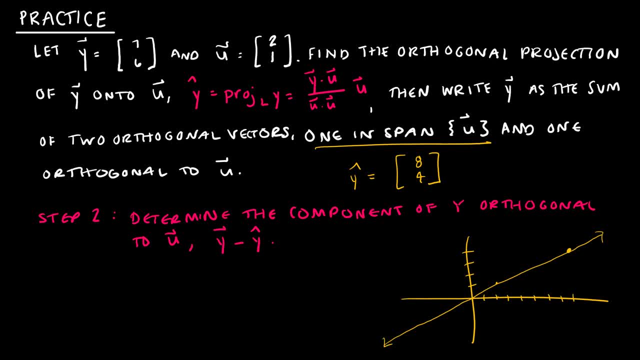 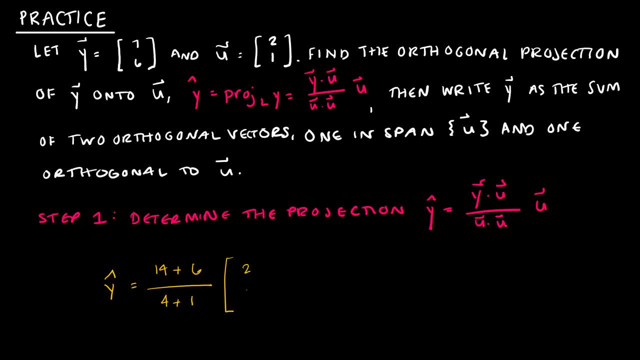 taken times vector u, which means I have whoops, I have 20 over 5 times vector u, which means 20 over 5 is 4 times vector u. So my projection is 8, 4.. So again, 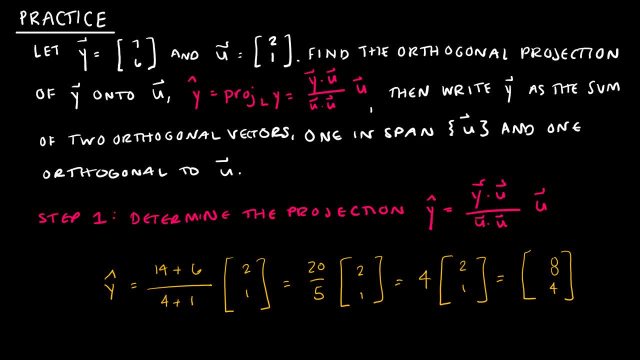 if you were to graph that, you would be looking at 7,, 6, and the line created by all of the scalar multiples of u, along the line created by 2,, 1, which obviously 8, 4 is on that line, And obviously 8, 4 is on that line And so that's going to be taken times vector u, which means 20 over 5, is 4 times vector u, So my projection is 8, 4.. So again, if you were to graph that you 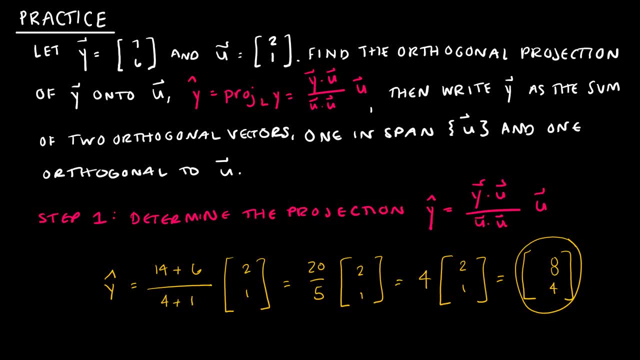 would be looking at 7,, 6, and the line created by all of the scalar multiples of u along the line. That is where y would sort of land if we were looking at the projection of y onto that line. Step two, then, is to find the component, which is what I would add to the vector that I just 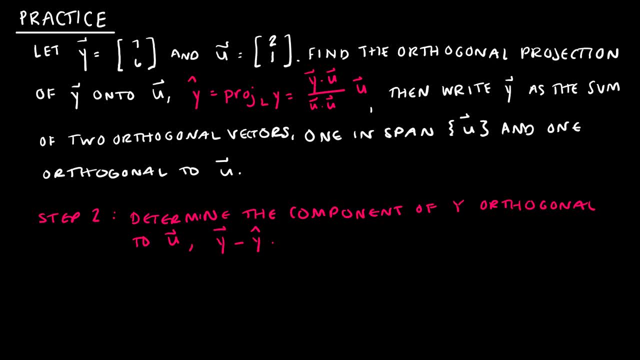 found in my last question, or last part of the question, so that I can write y as the sum of two orthogonal vectors. So one is in span u. Well, that's the one we just found. So, if you'll recall, I just found that the sum of two orthogonal vectors is the sum of two orthogonal vectors. 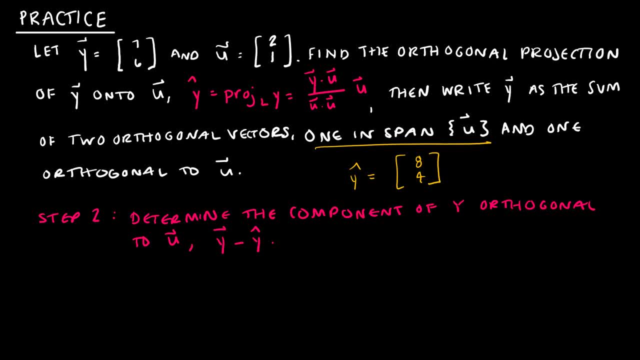 I just found that y hat was 8, 4.. And if I had a coordinate plane here- 1,, 2,, 3,, 4,, 5,, 6,, 7,, 8,- 1,, 2,, 3,, 4,, 8, 4 is out here And u was 2, 1.. So it's pretty easy to see and I don't have a ruler. 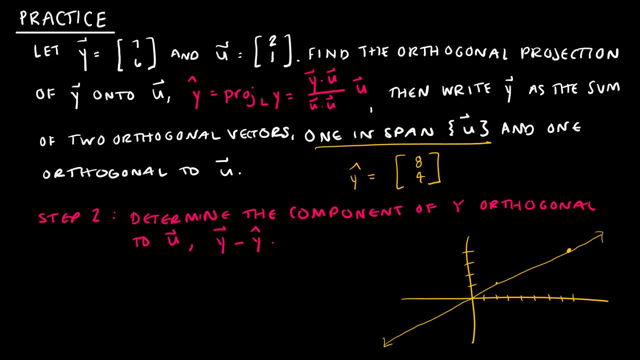 handy. but we can see that that line L, what I was looking for was the one vector. So I'm going to go ahead and do that And I'm going to go ahead and do that And I'm going. vector that was on the line, that's the one that's in the span of u, and certainly 8, 4 is in. 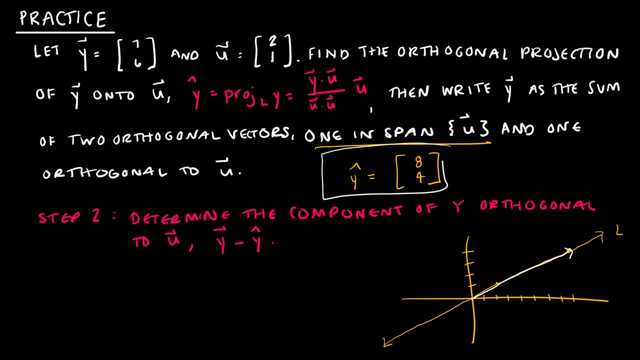 vector that was on the line, that's the one that's in the span of u, and certainly 8, 4 is in the span of u. And then I want to find one orthogonal to u, so at a right angle or perpendicular to u. 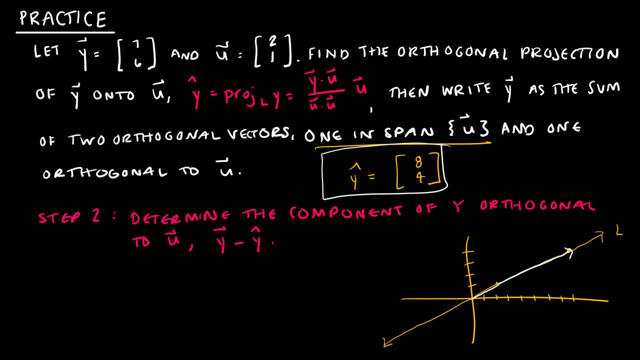 that would allow me to arrive at 7, 6.. So 7, 6 is about right here. So let's take a look. All I have to do is use this formula that says 7, 6 minus 8, 4.. So y minus y hat. 7 minus 8 is negative 1.. 6 minus 4 is 2.. So negative 1, 2.. 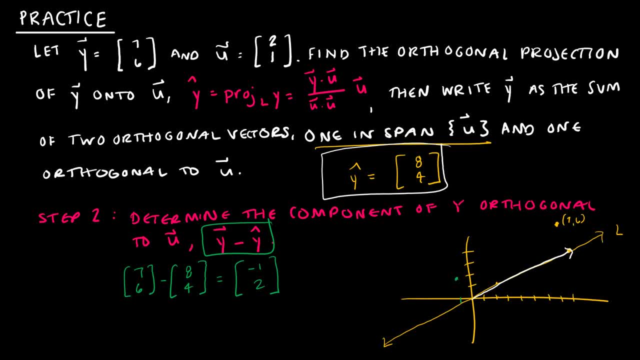 Now, if I think about the parallelogram rule, this makes perfect sense. So what I have found is the projection of 7, 6.. So 7, 6 is this guy. I have found that as the projection and the component that are, 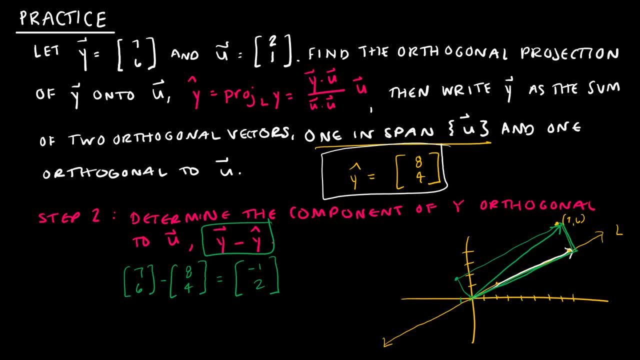 orthogonal to one another. So the question asks me to write y as the sum of two orthogonal vectors. so that sum would simply be 8,, 4,, which is the one that's in span of u, and then the one orthogonal to u, which is the one that's in the span of u, and then the one that's in the span of u. 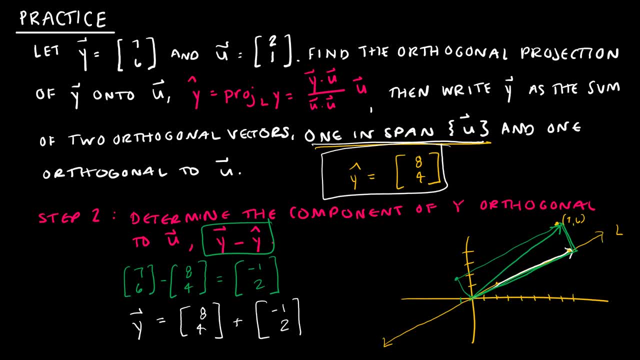 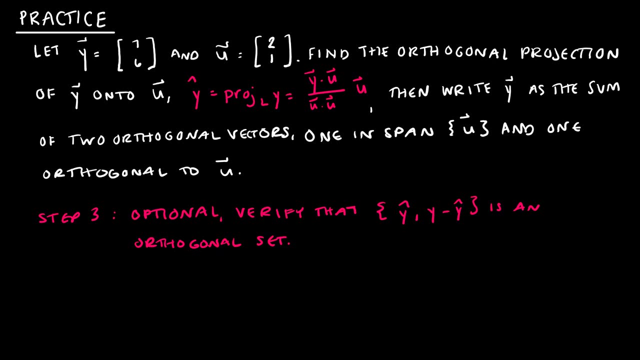 is negative, 1, 2.. And obviously I can check this by saying: 8 plus negative 1 is 7,, 4 plus 2 is 6, and that does get me back to y, The last part, which is completely optional, but if you want to check your work and you want to, 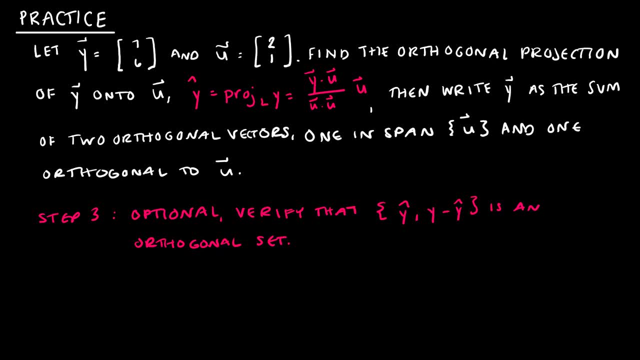 make sure that you did everything right. the last step is to verify that the set of vectors that we just came up with is in fact an orthogonal set, And that's the easiest part. So we have already done all of the hard work to find the projection, which is 8, 4.. And then we already found that y. 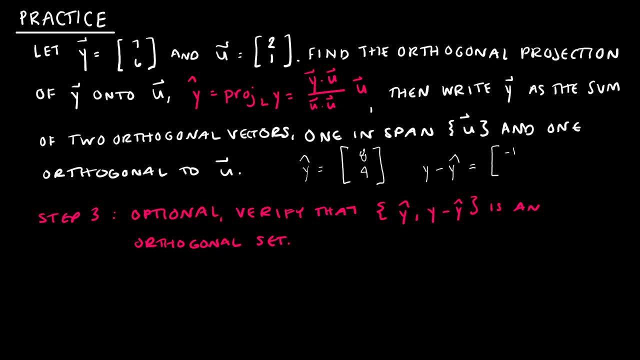 minus y hat is negative 1, 2.. And we know how to see whether or not something is orthogonal. We're just going to find the dot product. So I'm going to take the inner product of y hat and then of course the difference y minus y hat, which means I'm going to take 8 times negative 1,. 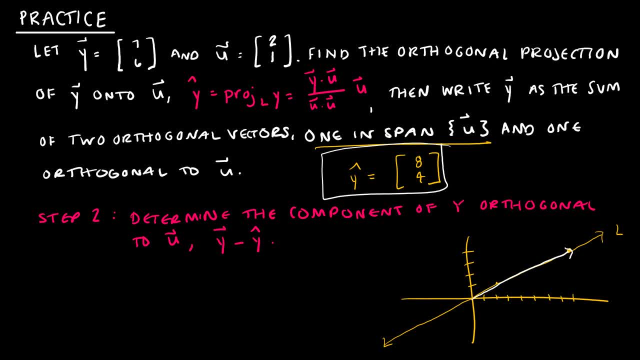 the span of u, And then I want to find one orthogonal to u, so at a right angle or perpendicular to u, that would allow me to arrive at 7, 6.. So 7, 6 is about right here. So let's take a look. All I have to do is use this formula that says: 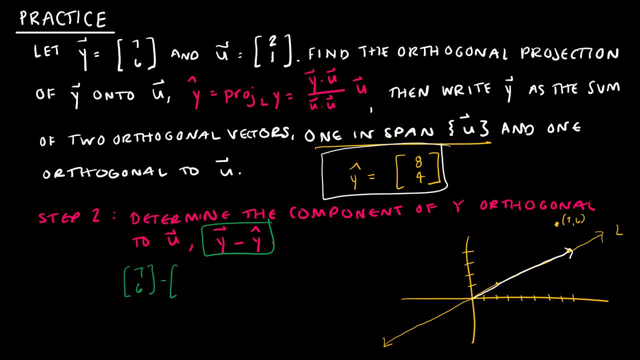 7,, 6 minus 8, 4.. So y minus y hat. 7 minus 8 is negative 1.. 6 minus 4 is 2.. So negative 1, 2.. Now if I think about the parallelogram rule, this makes perfect sense. So what I have found? 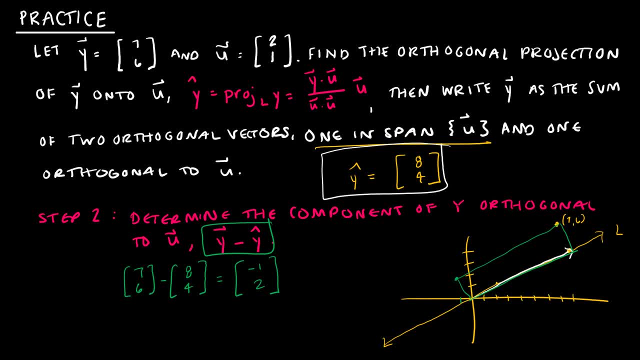 is the projection of 7, 6.. So 7, 6 is this guy? I have found that as the projection and the component that are orthogonal to one another. So the question asks me to write y as the sum of two orthogonal vectors. 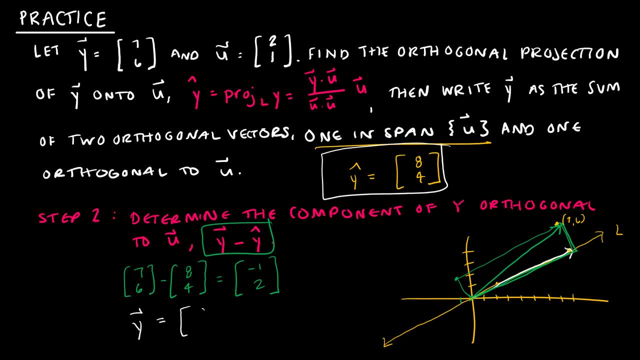 so that sum would simply be 8,, 4,, which is the one that's in span of u, and then the one orthogonal to u, which is the one that's in span of u, and then the one that's in span of u. 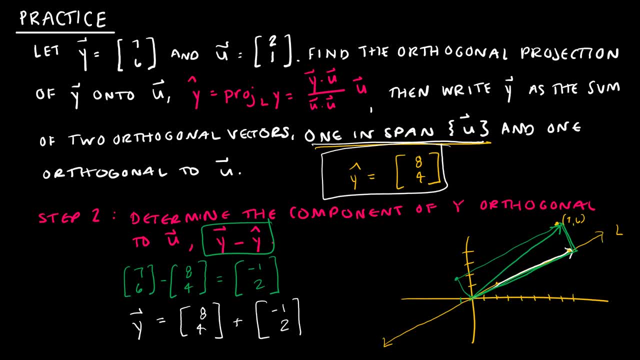 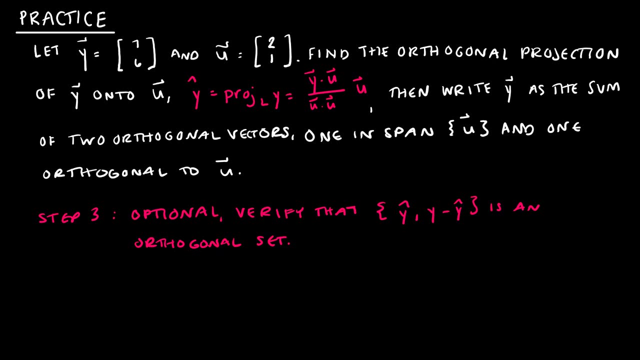 is negative, 1, 2.. And obviously I can check this by saying: 8 plus negative 1 is 7,, 4 plus 2 is 6, and that does get me back to y, The last part, which is completely optional, but if you want to check your work and you want to, 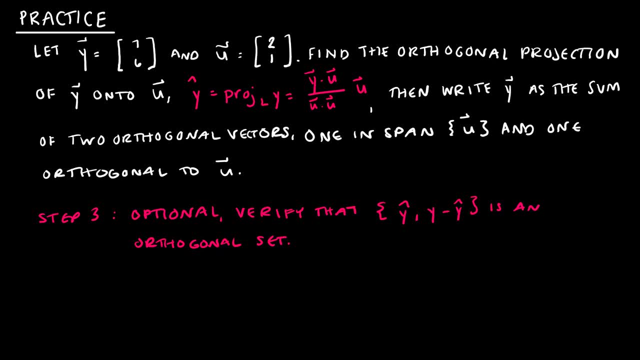 make sure that you did everything right. the last step is to verify that the set of vectors that we just came up with is in fact an orthogonal set, And that's the easiest part. So we have already done all of the hard work to find the projection, which is 8, 4.. And then we already found that y. 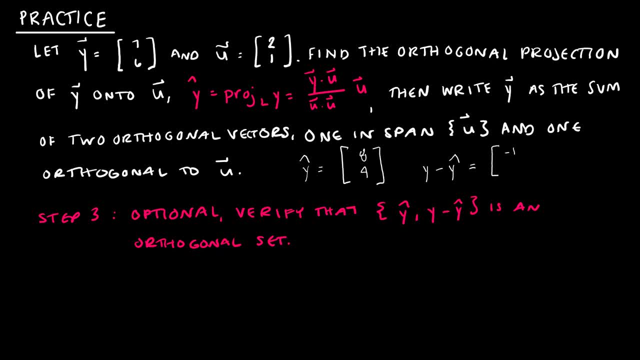 minus y hat is negative 1, 2.. And we know how to see whether or not something is orthogonal. We're just going to find the dot product. So I'm going to take the inner product of y hat and then of course the difference y minus y hat, which means I'm going to take 8 times negative 1,.